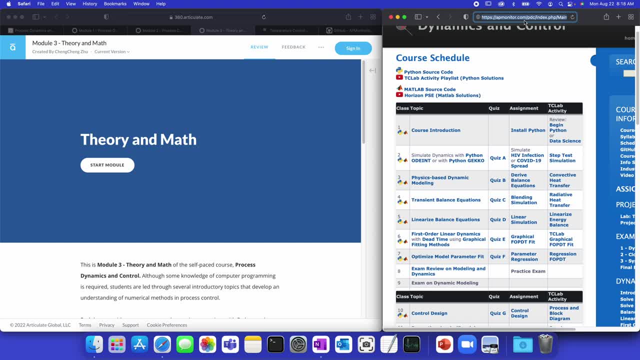 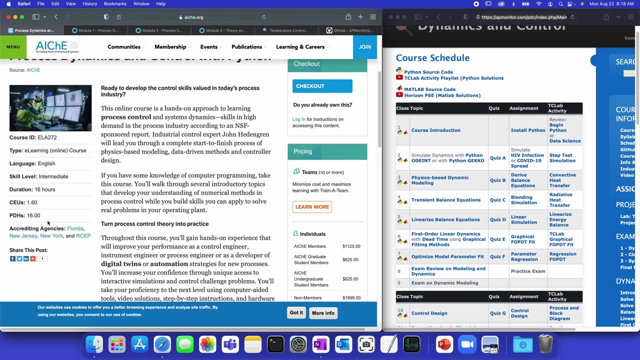 download it. It's also available freely from apmonitorcom. Just go to the courses and you'll see the Process Dynamics and Control course. Or if you want to take it through AICHE, then there are professional development hours that are available, as you can see right here. 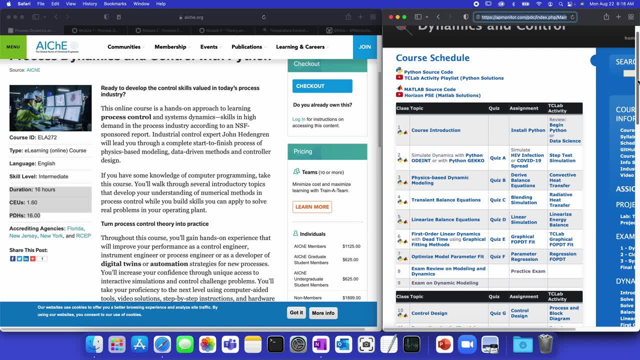 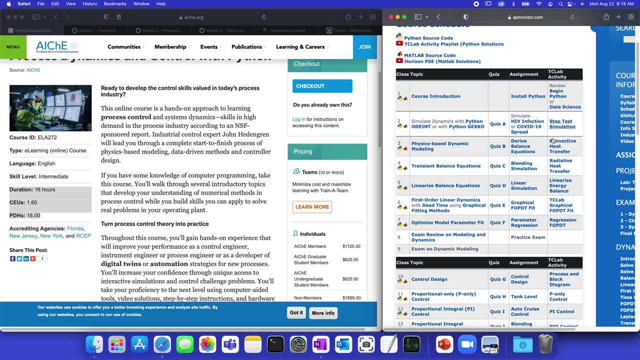 Okay, so let me go to the freely available course here on the right. It shows the different topics, the quizzes, assignments and then TC lab activity, the hands-on lab that goes along with each of the assignments. Now, here you'll see quizzes. For example, you can just select it from the web browser. 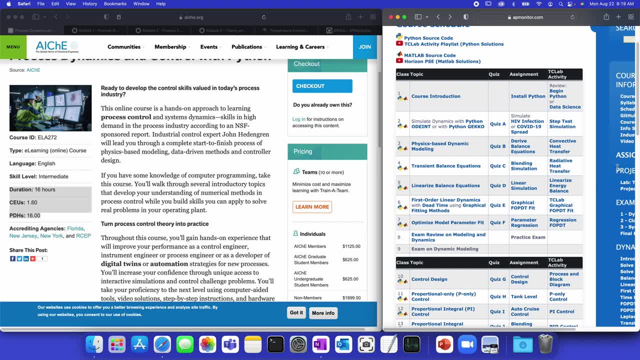 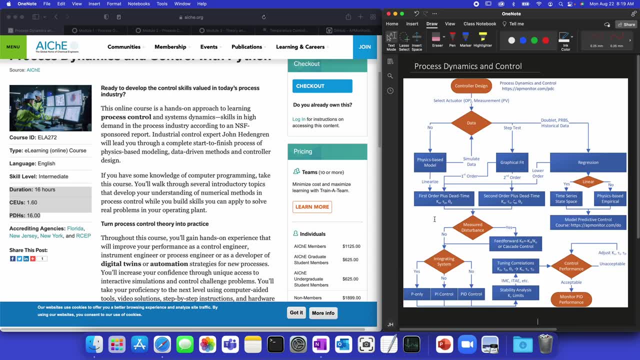 There's no login And you can take it at your own pace or visit the modules that you like. Let me go to just an overview of the course and talk about how these three modules are available. The first one is about Process Dynamics. We're going to cover the top portion of this course- flowchart. 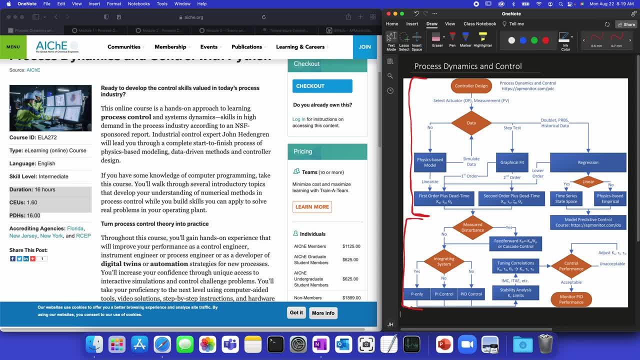 And then for the Process Control. it's going to be the bottom half where we develop controllers. Now the third part is the theory behind it. So more of the math that goes into the Process Dynamics and Control. So let's come to the process dynamics. 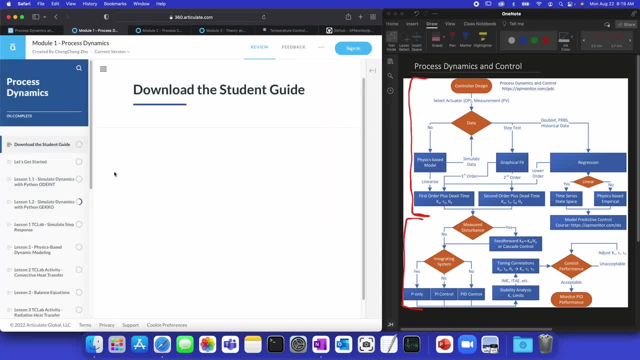 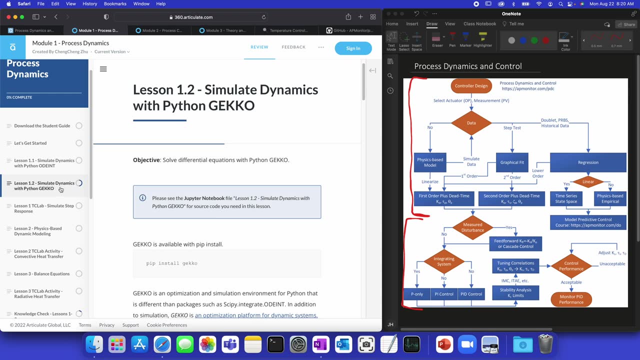 Let's go to the first module here. If we click Start Module then you'll see the different topics that are here. So the very first thing we're going to do is learn how to simulate dynamics, either with Python ODEint or Python Gecko. 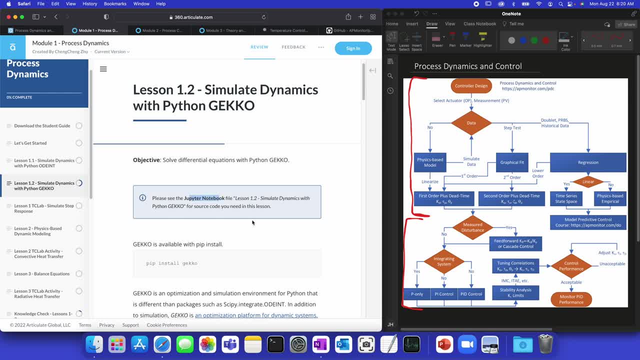 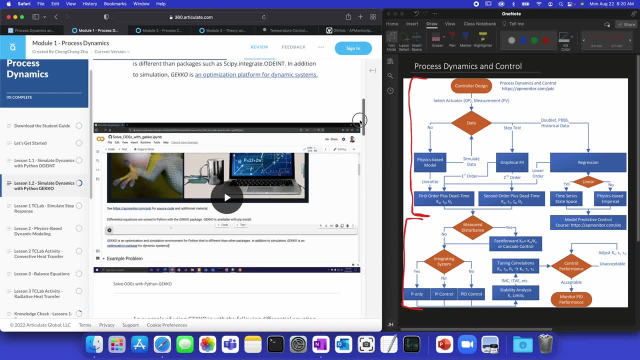 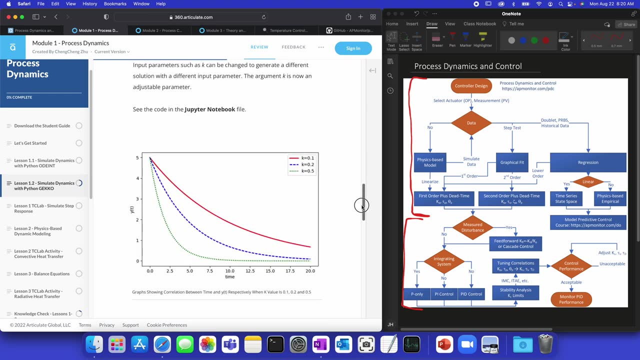 And you'll see Jupyter Notebook files that are available with each of these, with instructions on how to get started and videos to help you along the way. Okay, so we'll see exercises and examples And then we'll see some of these exercises here where it can help you get started. 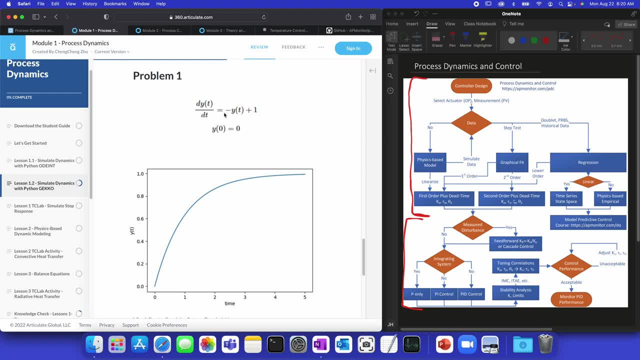 Here's a first problem. Solve this differential equation subject to initial condition equal to zero, And then you'll see the solution and the graph if you keep coming down. Okay, I'll select problem two And, similar to the first one, we're going to solve this problem. 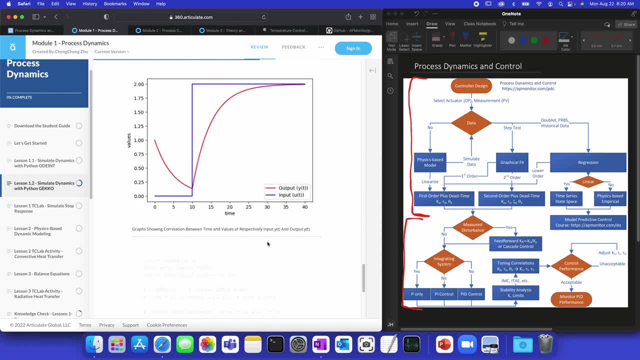 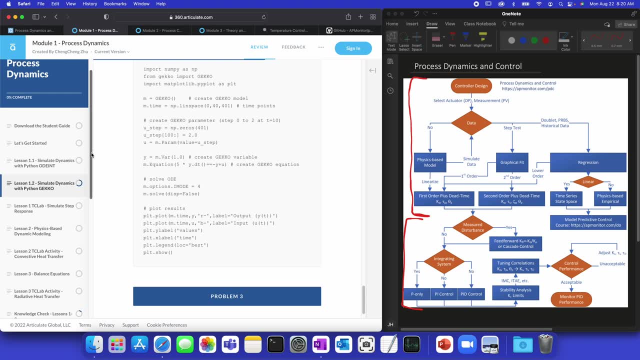 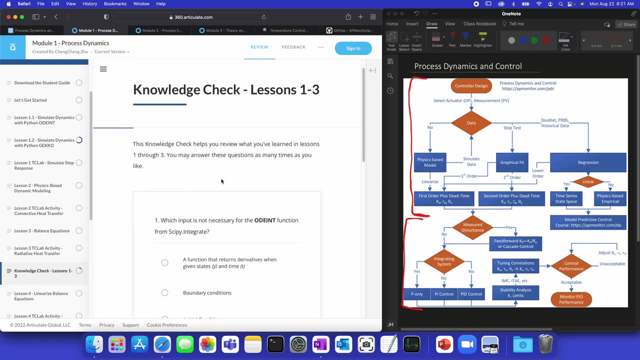 And if you need help you can click See Solution with the solution down below. All right, And at certain points in the course you'll also get to knowledge checks. Now knowledge checks will help test your knowledge, see where you are with your understanding of the content. 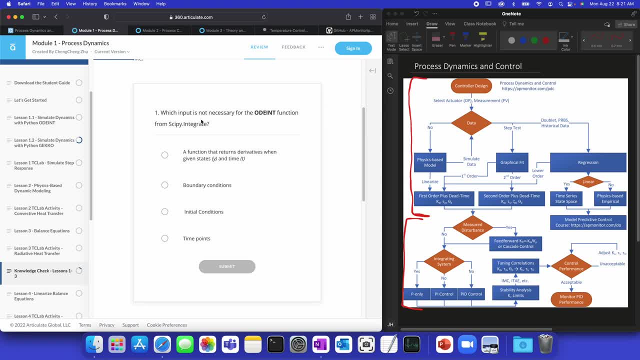 All right. So which input is not necessary for the ODEint function from scipyintegrate? And if we select the correct answer and click Submit, then we'll get feedback that it is correct. And if we select the wrong answer, then it will give us some feedback on why it's incorrect. 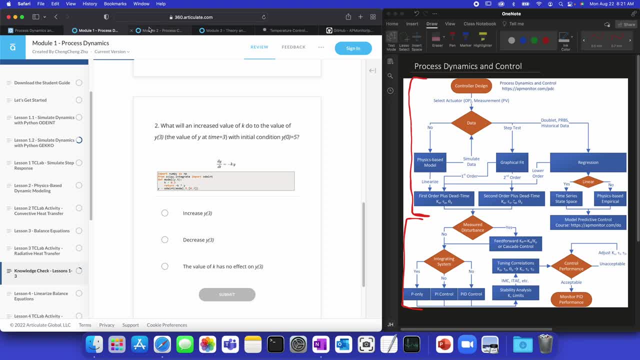 Okay, we can go down through these quizzes and other knowledge checks. So if you feel like you know a section, you can just scroll down through the lessons More quickly and then just take the knowledge check and then proceed through the course. It's self-paced exercises. 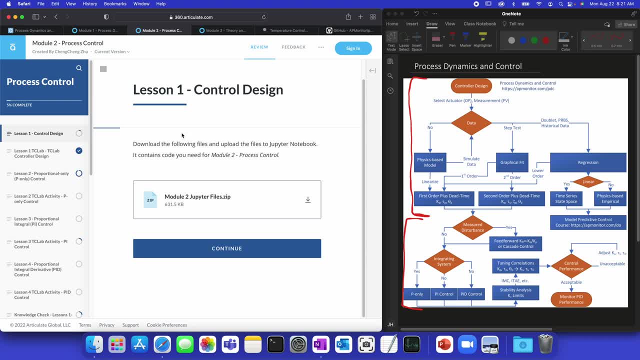 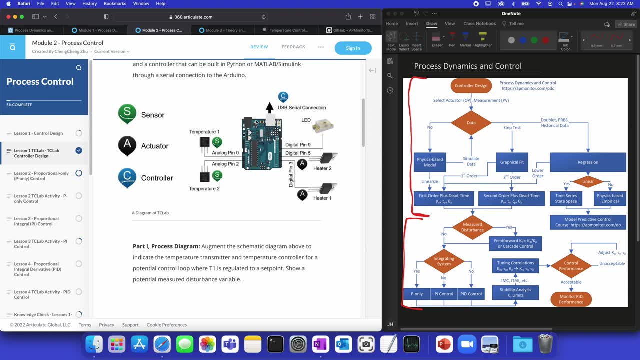 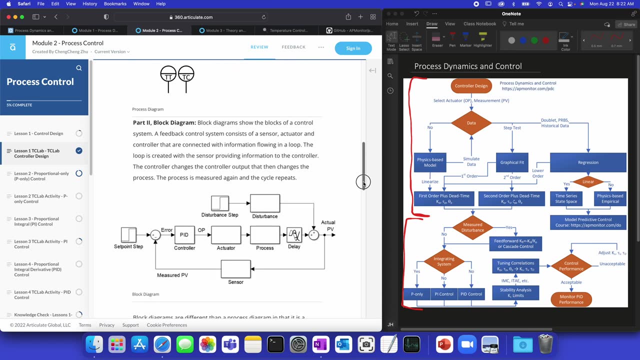 Okay, this is our process control module And I'll click Resume here. We're going to come here to the Temperature Control Lab And this is our device that we're going to use to run many of the exercises. It gives a little bit more description about it and somewhat about block diagrams. 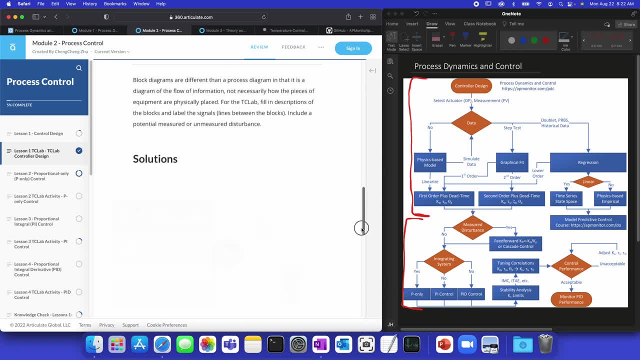 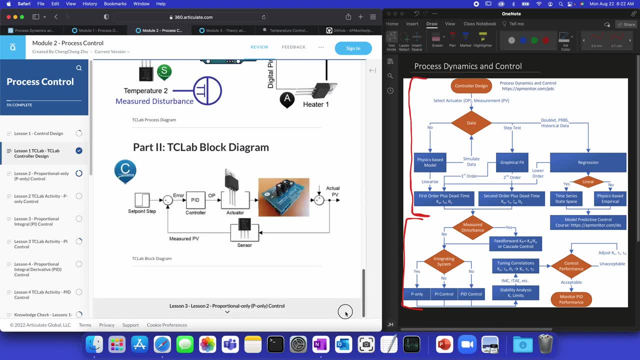 And how they can show the flow of information. And then we're going to do the same thing with this Temperature Control Lab. Okay, and we'll show it in practice. So, really, the Temperature Control Lab is taking the theory and the methods and then showing how they apply on a real problem. 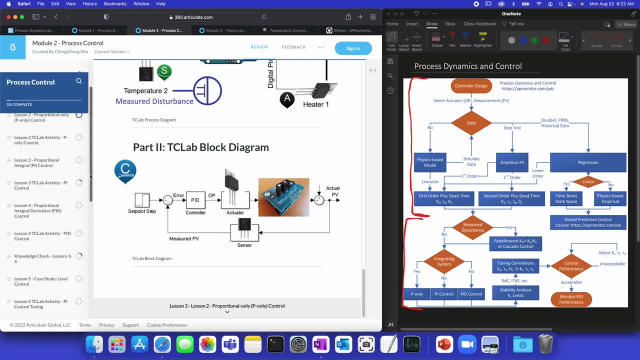 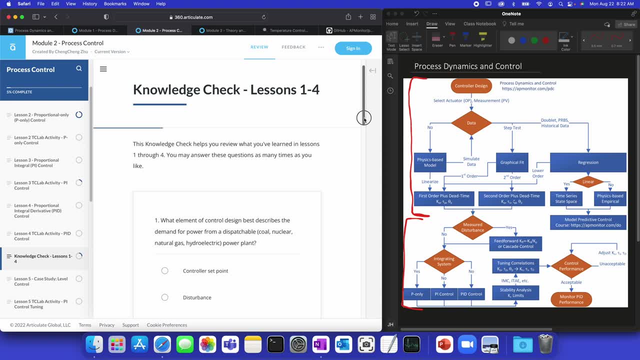 You'll also have knowledge checks in this one as well. I'm going to come to Lesson 1-2.. All right, so we would select here from what element of control design best describes the demand for power from a dispatchable such as coal, nuclear, natural gas, hydroelectric power plant. 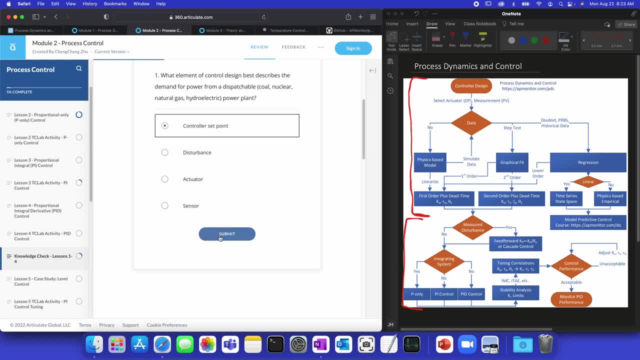 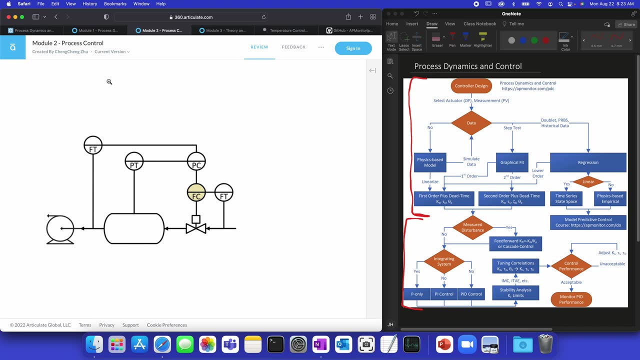 So we want to try to meet that demand. So that would be our controller set point. All right, and if I come down here, we'll see what is not a role of the flow controller. So the one that's highlighted right here, which is the flow controller. 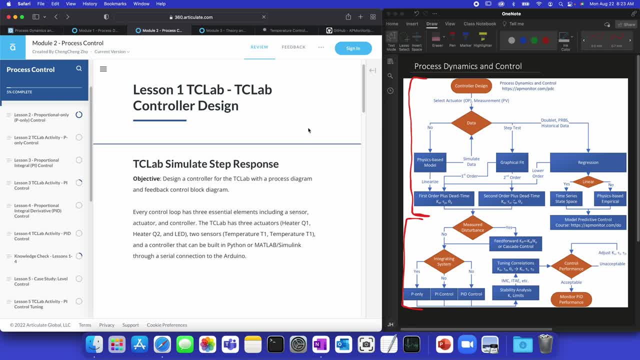 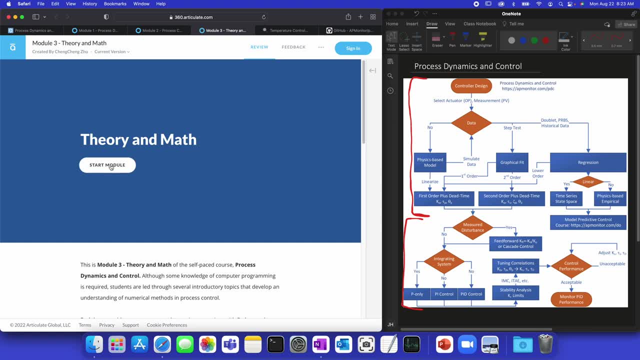 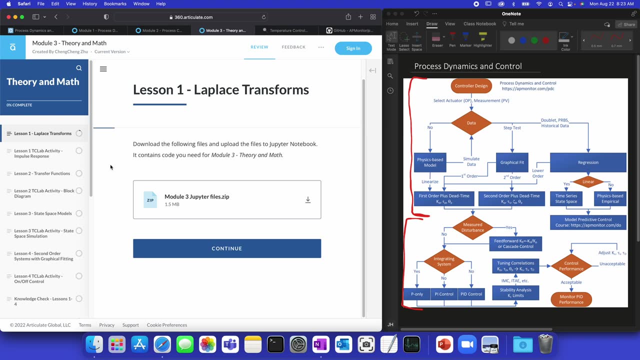 Okay, and then I can select that answer and move on. I'll show you also module number 3.. This is the theory and math behind many of the methods. Okay, we've broken this out, in particular because the first two modules are very hands-on, very practical. 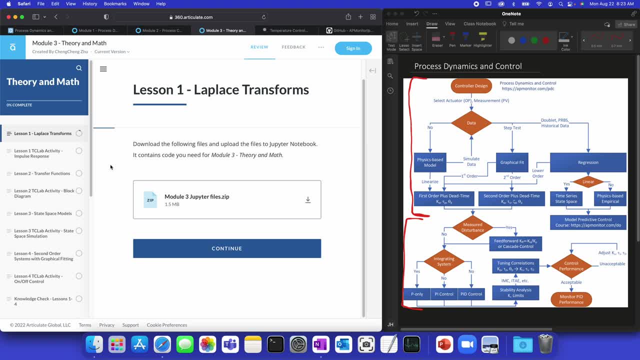 And then, for those that are interested, this one talks about things like Laplace transform, state-space models or derivation. It gets into some more advanced topics like second-order systems, graphical fitting, regression and other topics like stability analysis. Okay, so there's the overview. 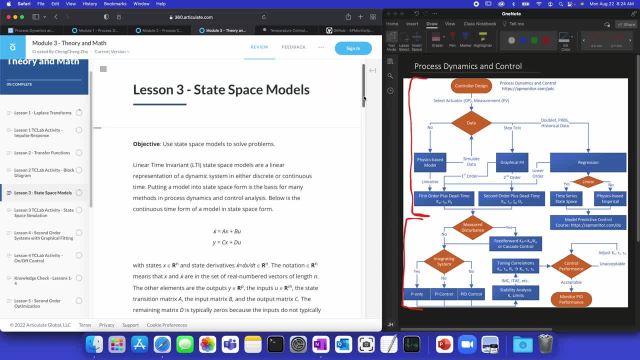 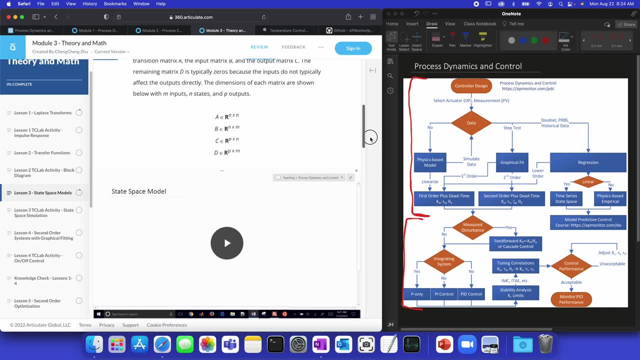 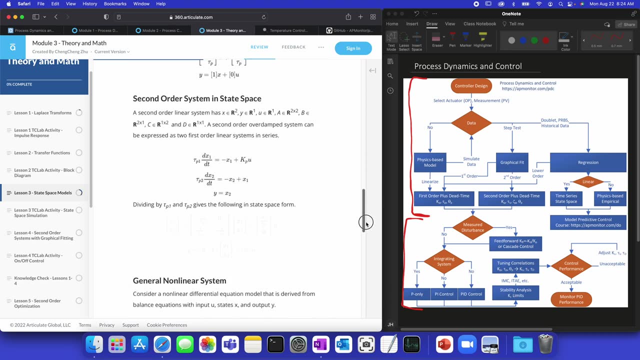 I'll go to, for example, state-space models. It'll give an introduction to state-space for multivariate system identification, modeling and control, And then we'll talk about things like stability analysis and nonlinear systems, for example. Here you'll also have other knowledge checks. 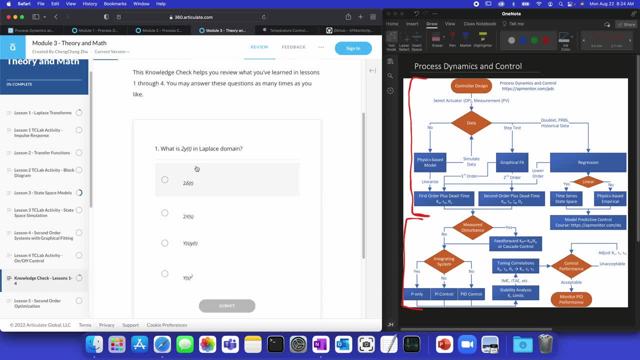 Okay, so here's something 2 times Y of T in the Laplace domain. It would be this one, And we'll click Submit And it'll give us some feedback. Now again, if you don't get it right, you can select Take Again. 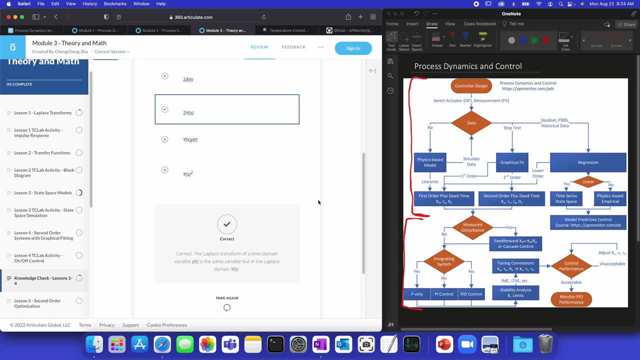 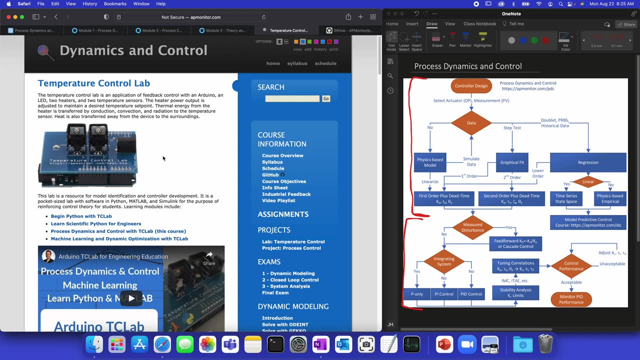 and then you can select the correct answer. Okay, so that's the course overview. Again, if you want to do this yourself without going through the AIC at Chia course, it is available. You will need to get a temperature control lab. 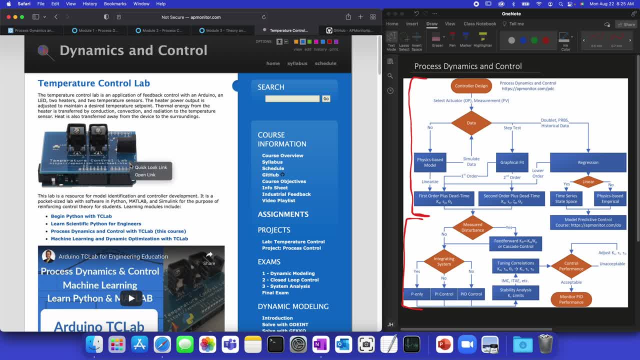 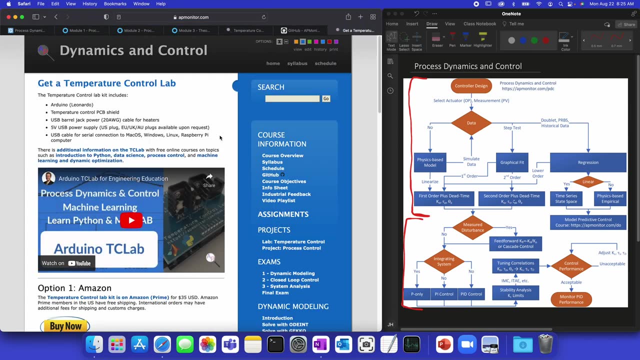 It's available from this link right here. My browser even recognizes this link, It looks like, And so if you open that up, you can come here and then get a temperature control lab, get TC lab, and you can get it from Amazon or a couple other sources. 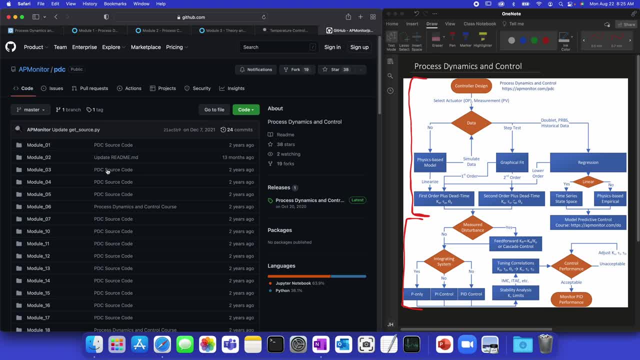 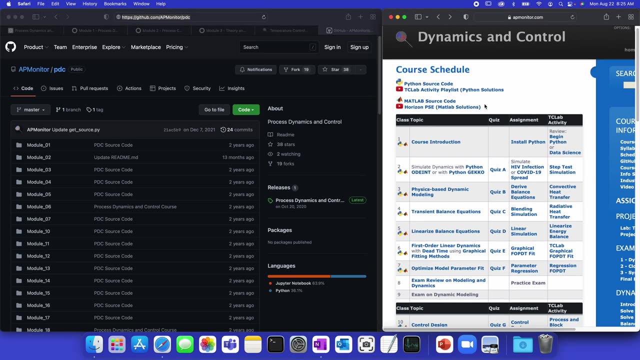 Okay, and then I'll just come back here to the GitHub repository as well. All of the files, the source files, are available here. And I'll show you one other thing for those that want to use MATLAB, So for MATLAB users, there is also MATLAB source code available. 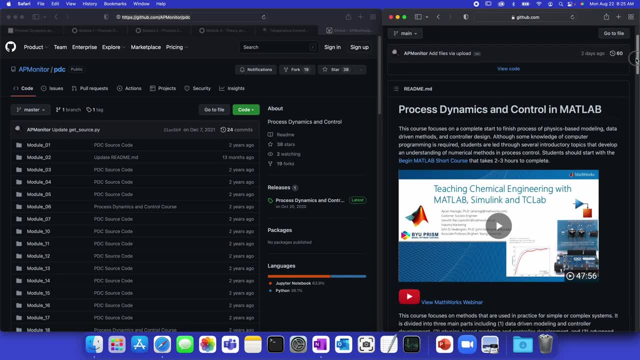 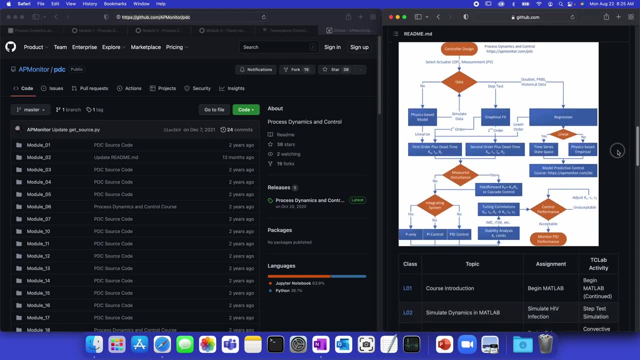 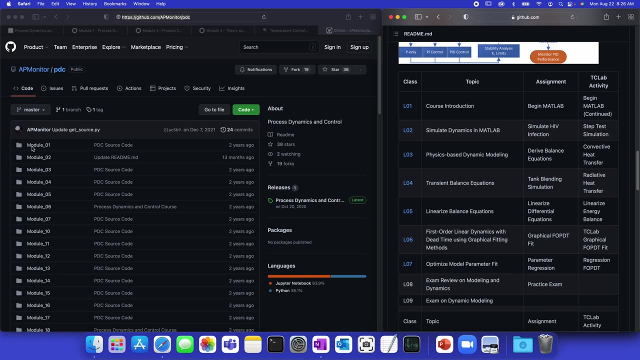 This one is highlighted from this MathWorks webinar. We talked about teaching chemical engineering with MATLAB, Simulink and TC lab, And you'll be able to see all of the equivalent modules. So here L01 is Module 1 on down. 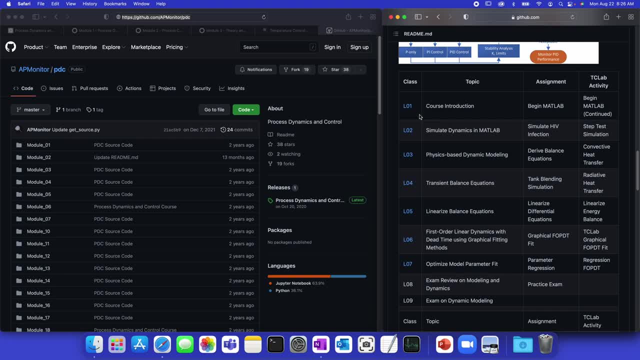 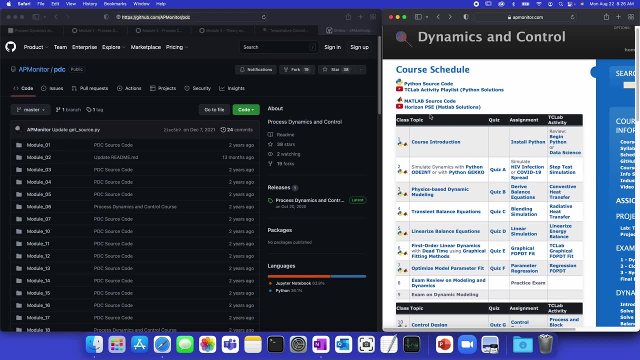 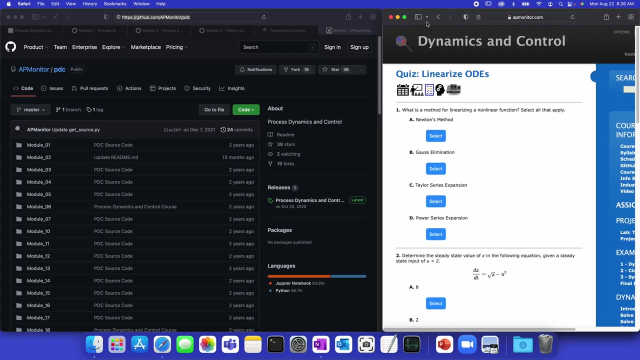 So all of this is also in MATLAB Live scripts and Simulink, if you'd like to go through the course that way instead- And again, these are the topics that are available- Online quizzes here that you can do similar quizzes through this online web browser without logging in. 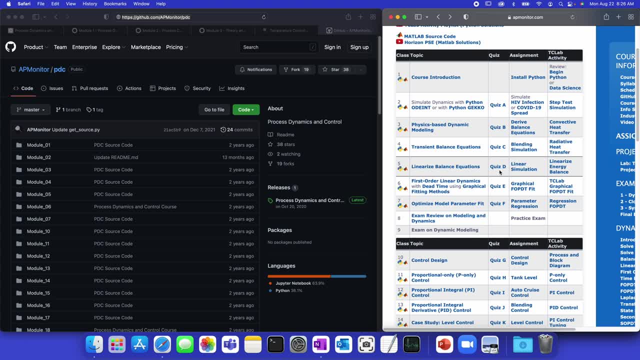 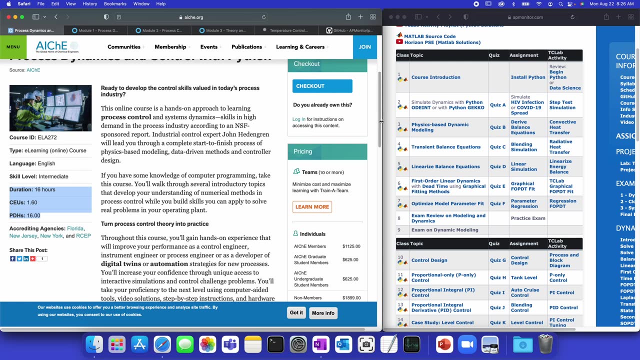 You won't get a continuing education credit or things like that, but the content is available here if you'd like to access it Through the apmonitorcom website. Well, I hope you enjoyed this course overview And I'd definitely like to hear your feedback on these modules. 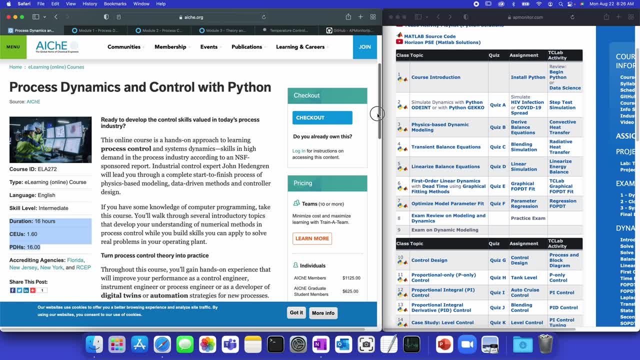 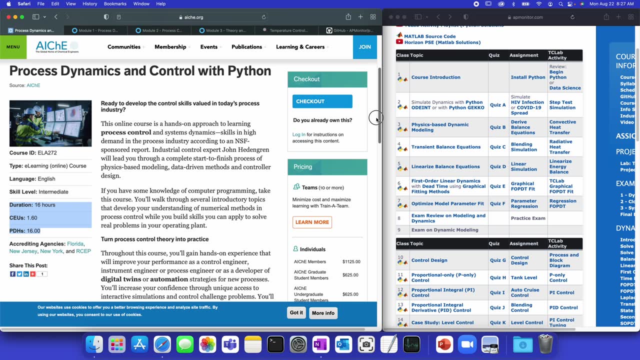 I really appreciate the staff from AICHE, for especially the instructional designers, for what they've done to take this content and make it available for continuing education, professional development. I know that I've had many that have requested it, Many that have requested that this content that we have on the website. 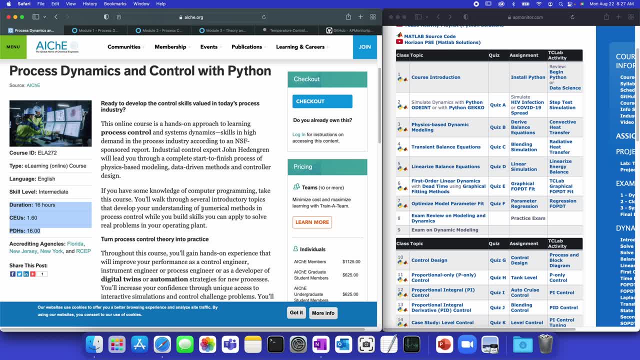 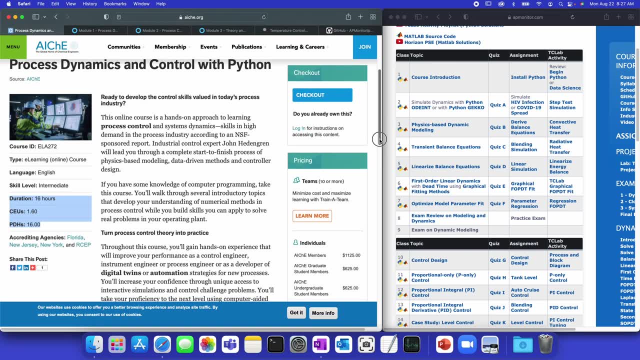 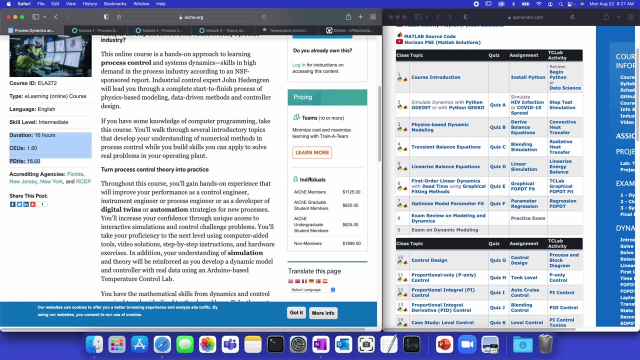 be available with some type of certification or credit option. So this is available and it's available to AICHE members, graduate student members, undergraduates or non-AICHE members as well, as you'll see over here on the right.